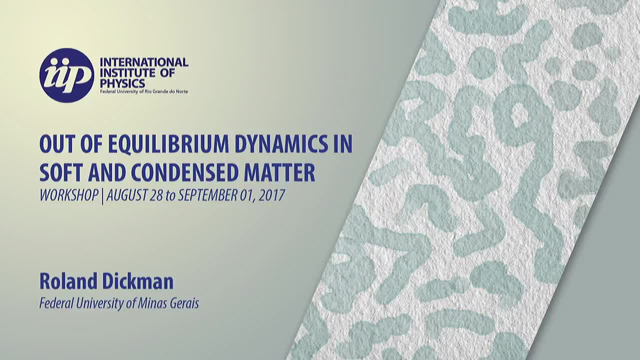 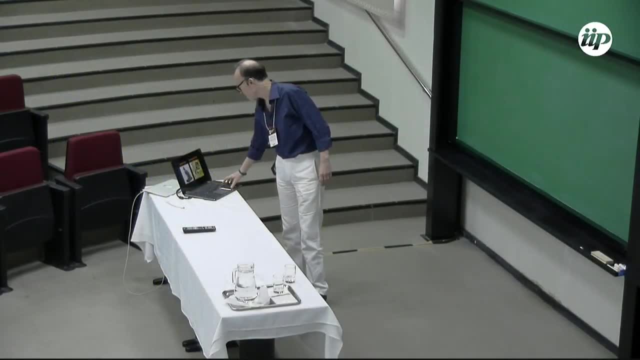 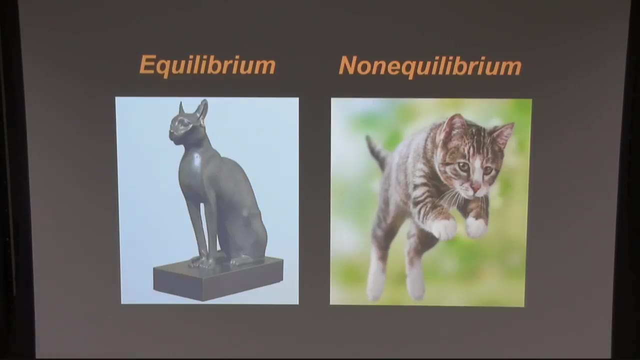 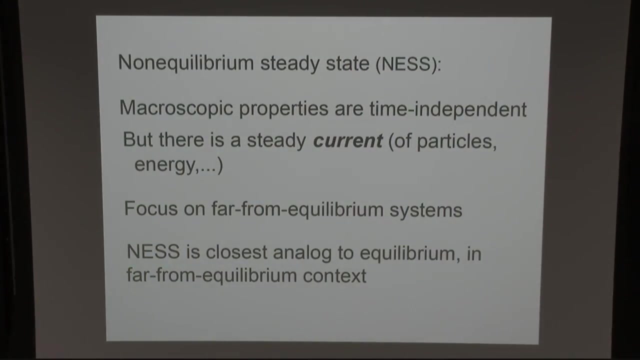 Oh, I don't get the gadget. Okay, I have to do it by hand. So I'm going to talk about these topics very fast, because there isn't much time. So look, equilibrium is beautiful, elegant, ancient, dead, and non-equilibrium is everything else. But I'm going to talk. 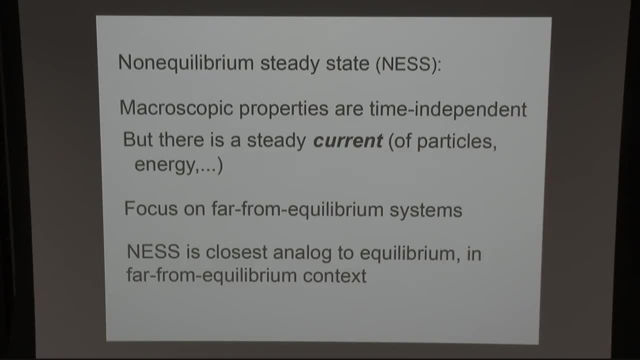 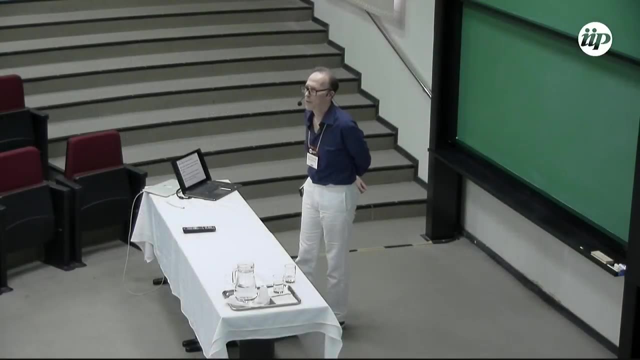 about non-equilibrium steady states, which is sort of in between. Of course they're characterized by currents in the system, So they are systems that are out of equilibrium. They can be quite far from equilibrium, but the macroscopic properties are time-independent. 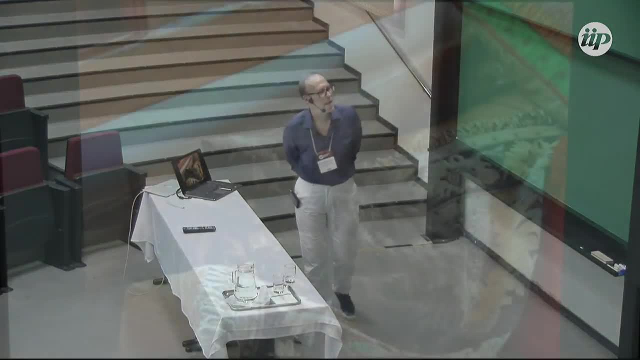 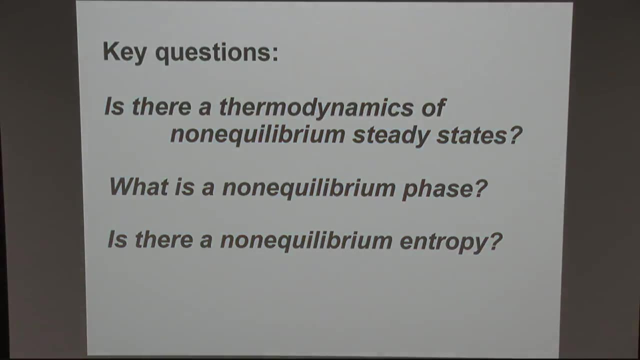 So it's a bit like this situation: The cat is alive and happy and almost sleeping, but it's still far from equilibrium. So the questions I want to ask are whether it's possible to develop current. So what is a non-equilibrium phase? I'm not going to answer that, but I'm going to show. 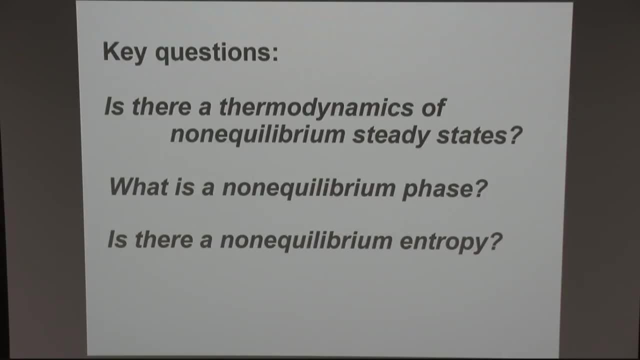 you that there are some problems associated with this question. And finally, if it's possible to define a non-equilibrium entropy. And all of this will be done in the context of simple stochastic lattice gases, which I will use in a few minutes. So I'm going to start with. 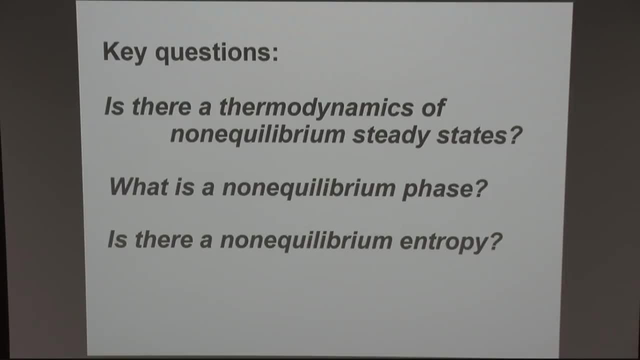 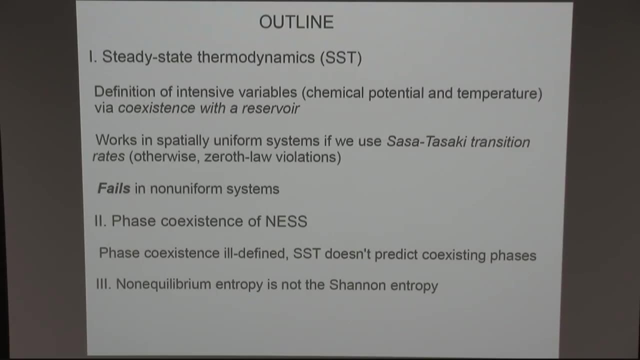 a state-of-the-art analysis. It's been done with shallow星 systems of several types of thermodynamics, The tteokbokki data that we use as experimental systems to test these ideas. So first I'm going to talk about steady state thermodynamics, In particular. the question 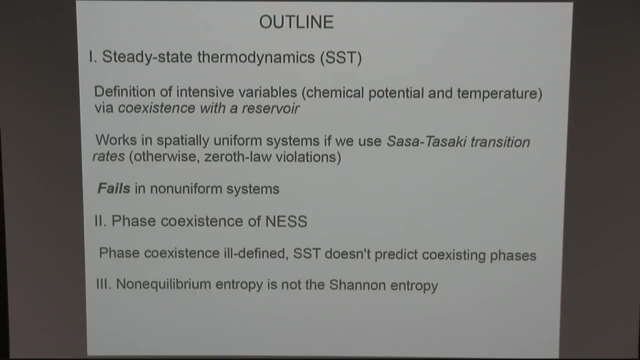 of defining intensive variables like chemical potential or temperature for non-equilibrium steady states, And this will be done via the idea of coexistence with a reservoir. We have a reservoir which is an area of theceğiz z yaw ie we call it a reservoir of solid. 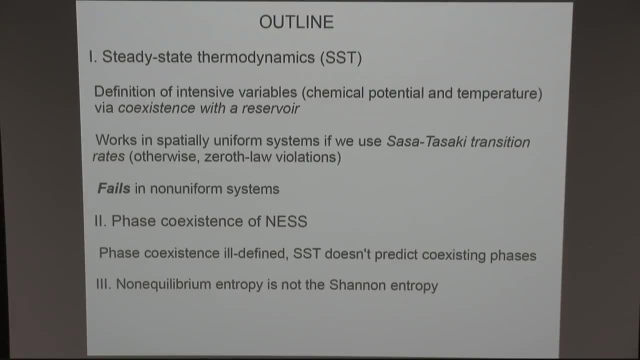 materials with defined properties, like a defined chemical potential, and we look at what happens when the reservoir can exchange particles, for example, with the system that's in a non-equilibrium steady state. We can use that as an operational definition of the chemical potential. 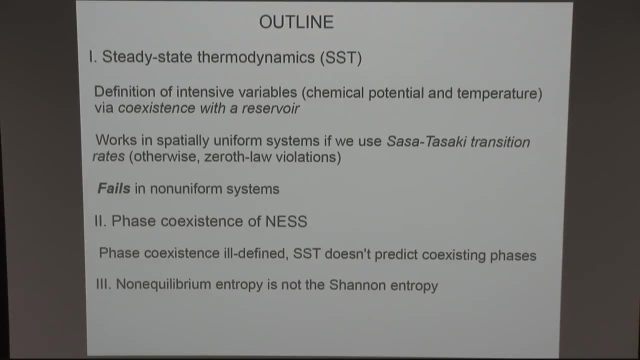 but then we have to ask if this definition is consistent in the sense of the zeroth law. So we'll look at that. Then I'm going to talk a bit about phase coexistence within non-equilibrium steady states and finally talk about this last item that we'll see at the end. 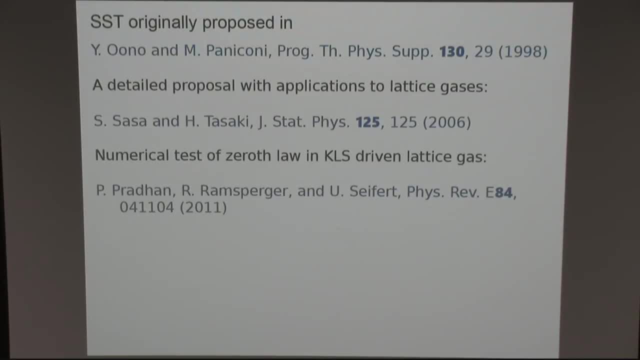 So, very briefly, the idea of steady state thermodynamics was proposed by Ono and Panicone some 20 years ago and there was a detailed proposal for applications to lattice gases and other things like that, Other systems by Saza and Tazaki and, more recently, a test of the zeroth law in the driven lattice gas. 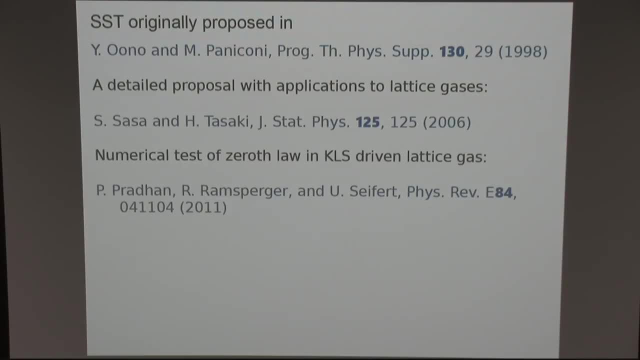 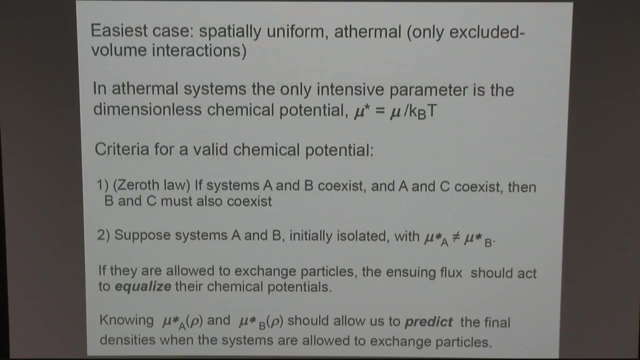 This last work is worth mentioning that these authors verified the validity of the zeroth law to within something like 5%, and they were more or less happy about that. I think 5% violation is very bad. It's a violation. I mean thermodynamics has to be exact. 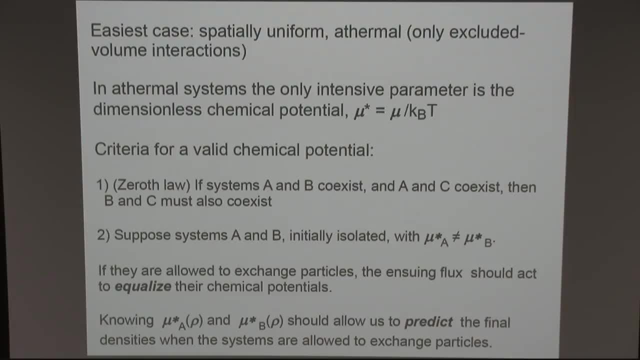 But the reasons for that violation weren't clear at that moment. So let's look at the easiest possible case, which is an athermal system. In other words, there were only excluded volume interactions between the particles, and in that case in a lattice gas at least. 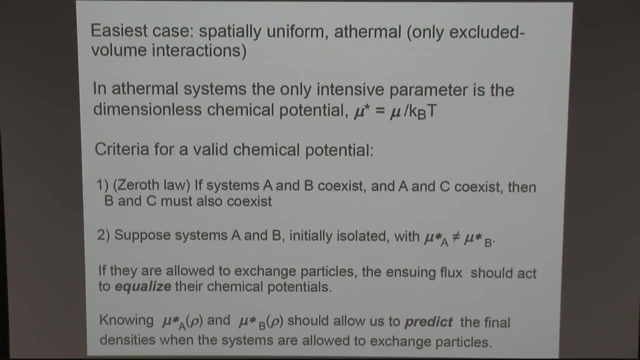 the intensive parameter of main interest would be the chemical potential. It's a dimensionless chemical potential, mu, scaled by kB T. And what do we want from a chemical potential? Well, of course, it should satisfy the zeroth law in the usual sense. 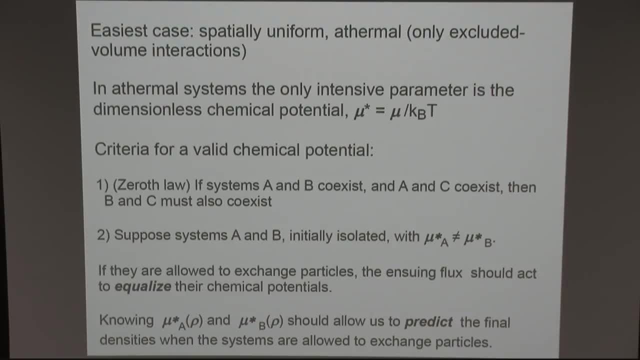 and it should have some predictive value. That is to say, if we start with two systems that are isolated and have different chemical potentials and we put them in contact, then we should be able to predict the final densities that these two systems come to. 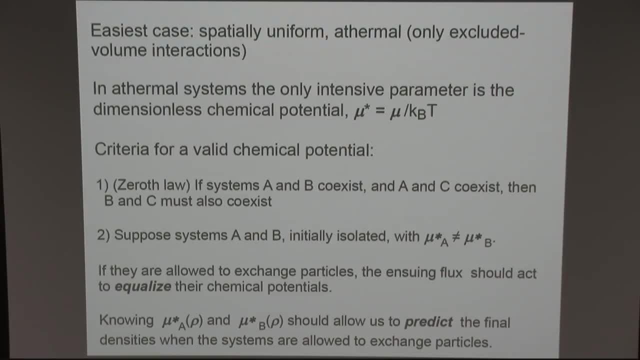 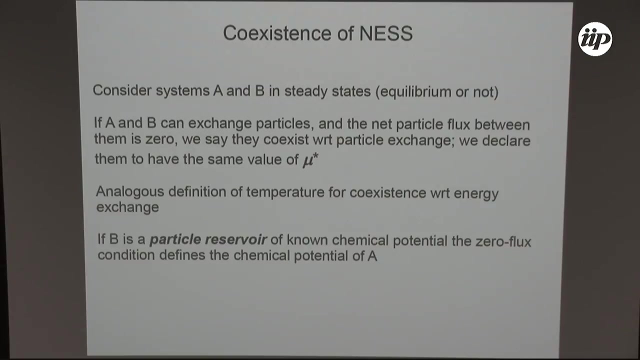 by equating the chemical potentials that hold for the isolated systems. I mean, if that's not true, then really what we're talking about as thermodynamics is not going to have much utility. Okay, so coexistence is simply the idea that if two systems are able to exchange, 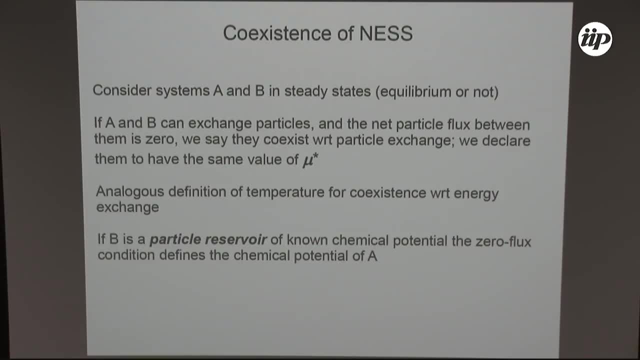 for example, a chemical potential, then we should be able to predict the final densities that these two systems come to. Okay, so coexistence is simply the idea that if two systems are able to exchange, for example, particles, and they reach a state in which the net flux of particles between them is zero, 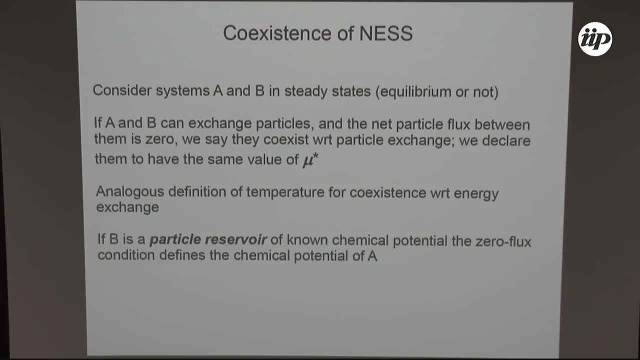 then we say they coexist. with respect to exchange of particles In equilibrium, we would say they're in equilibrium, they're in chemical equilibrium, but I won't use that to talk about non-equilibrium. Yes, Yes, Okay, but let's assume that everything goes through with short-range correlations. 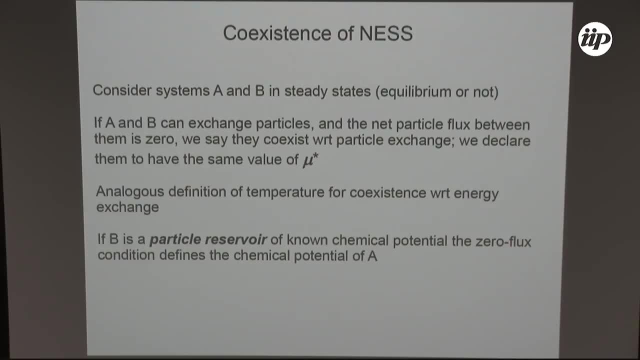 Okay, but let's see how it goes. It's true, but just thinking of macroscopic thermodynamics, this is the operational definition. So good, Now, in this context of coexistence, if one of the systems of interest is a reservoir with a known chemical potential? 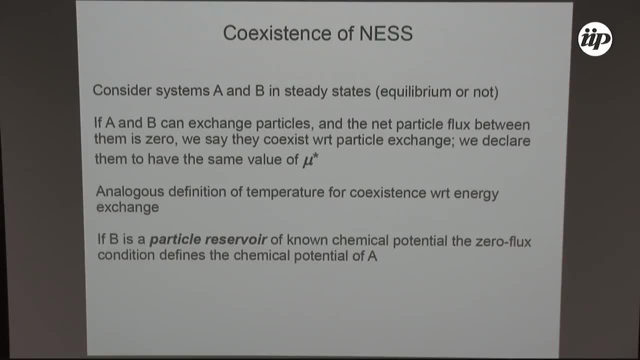 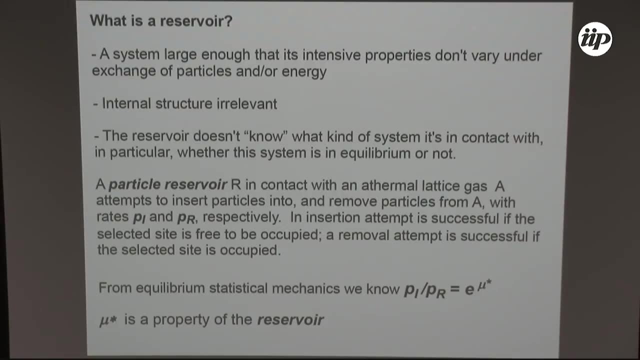 then we can use that to define the chemical potential of the other system, be it in equilibrium or in a non-equilibrium steady state, A reservoir. by a reservoir I mean simply a system that tries to insert or give a certain quantity to the system of interest and extract that same quantity with another rate. 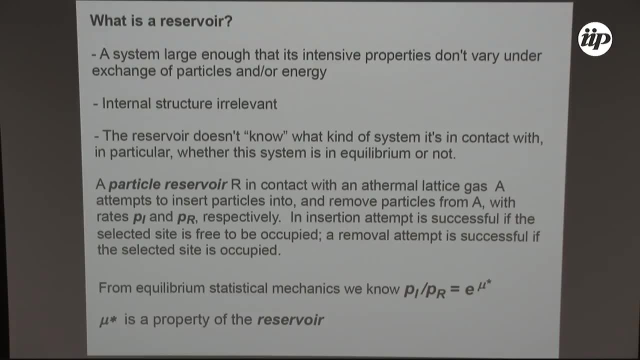 And what defines the chemical potential of the system is simply this ratio of the insertion attempt and removal attempt rates. So it's the ratio that's important and that's an intrinsic property of the reservoir. The reservoir doesn't know anything. It doesn't know anything about who it's interacting with, if it's an equilibrium state or a non-equilibrium state. 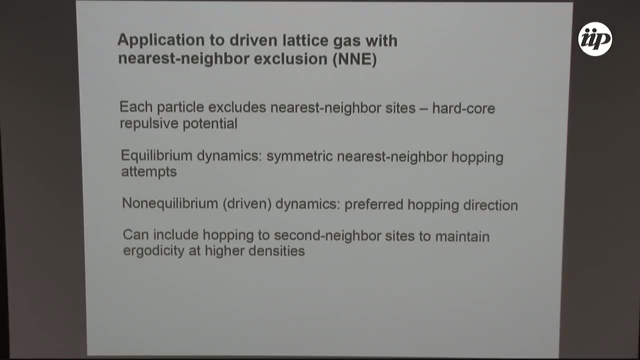 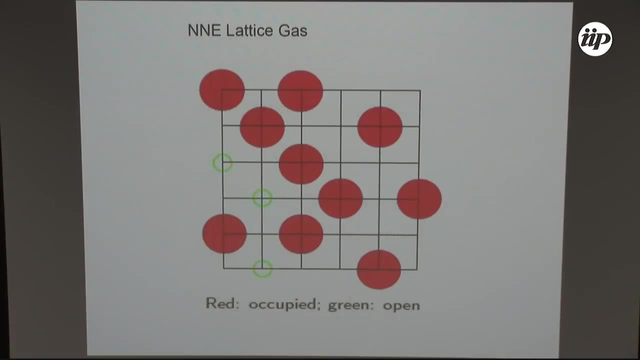 And now I'll apply this to a model that's simple but not completely trivial, which is the lattice gas with nearest neighbor exclusion. So a picture of what's going on is this: The big red circles are the particles that live, in this case, on the sites of a square lattice. 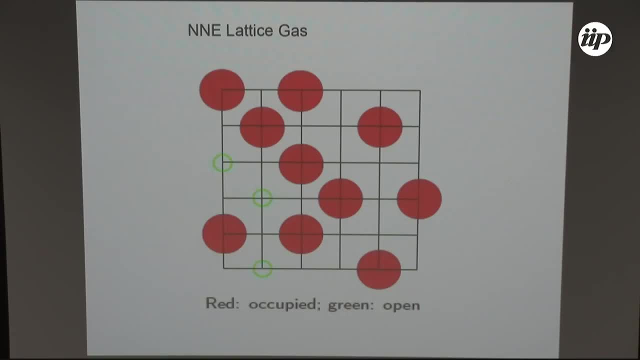 And the rule is that I can't have two nearest neighbor sites. They're occupied simultaneously. You see certain sites in green, circled in green. those are the sites where I could insert a new particle without violating the nearest neighbor exclusion condition. I'll call those open sites. 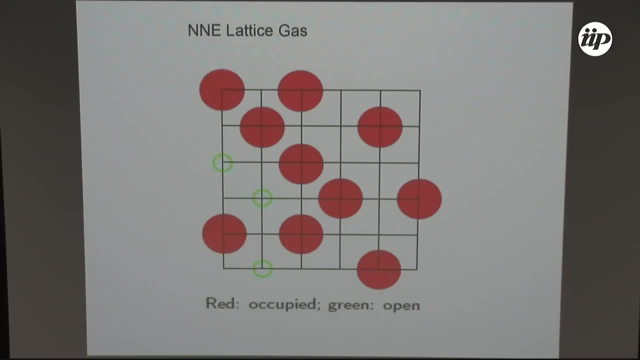 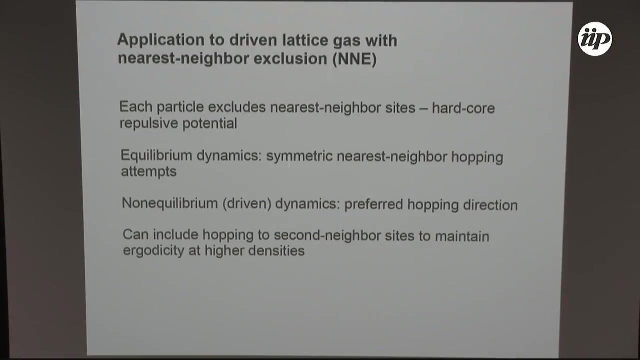 And if you think about this insertion and removal dynamics with a reservoir or with another system, you see that it's the fraction of open sites that are going to be important in defining the effect of chemical potential. So that's the model. It exists in an equilibrium version, which is a kind of lattice version of hard spheres. 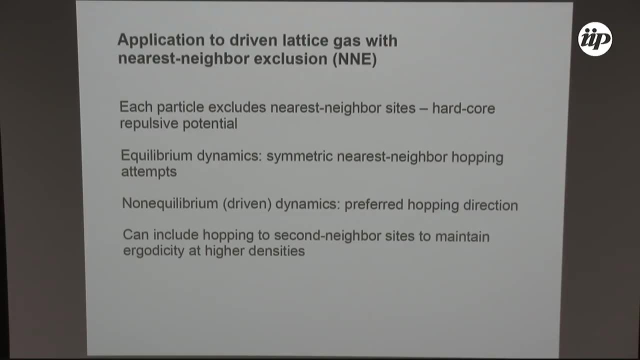 a model that was widely studied back in the 60s. And if you equip it with a dynamics, a hopping dynamics, then you have a dynamic lattice gas. And now you can do this. You can drive it by imposing a preferred direction on the hops. 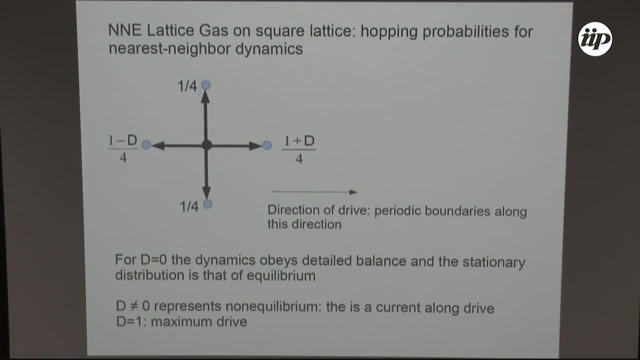 So I'll do that by introducing a parameter d. So for this case of only nearest neighbor hops, you see that when d is zero, I have symmetric hopping attempts in the four directions, And so we have equilibrium. When d is different from zero, I'm preferring one of the directions. 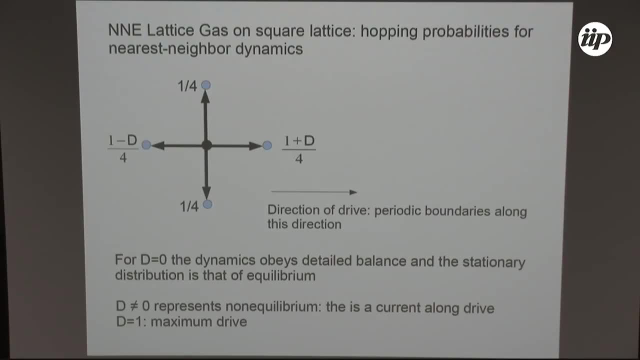 And that leads to a drive. Of course it's absolutely essential that you have periodic boundaries in this direction. In fact, in the studies I talk about there'll be periodic boundaries in both directions, unless otherwise stated. But you must have periodic boundaries along the drive. 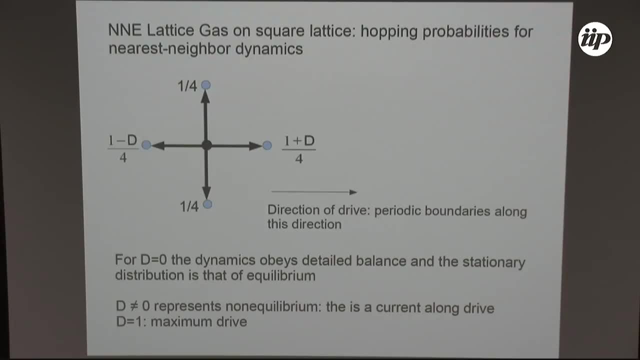 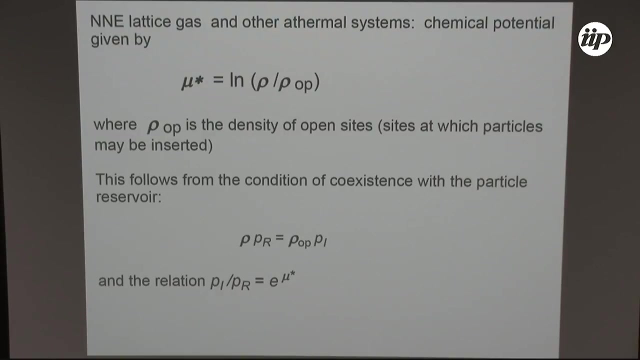 If not, you go back to having an equilibrium system in some sort of external field, So with periodic boundaries and d different from zero. you establish a steady current and the system relaxes to a non-equilibrium steady state. And now we can think about how the interaction with a particle reservoir will go. 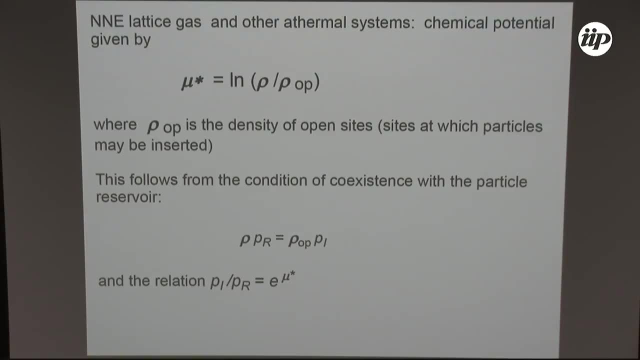 And remembering that relation between the insertion and removal probabilities and mu star, the chemical potential, you quickly reach this conclusion, which is valid. is valid in and out of equilibrium, where rho is just the particle density, the fraction of occupied sites, and rho op is the density of open sites that I mentioned. 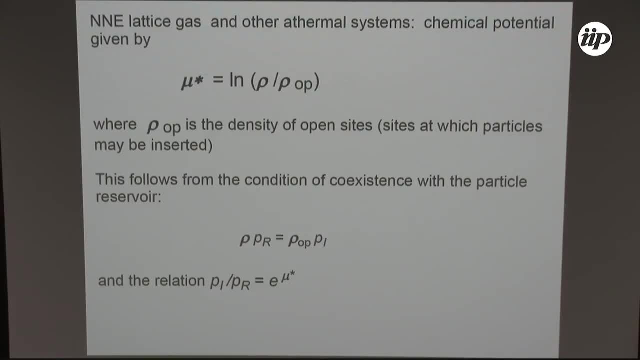 So to derive this relation of coexistence, you need to assume that the two systems that are exchanging particles are statistically independent. So from that point this implies a slow exchange limit because I need to have between any pair of subsequent exchange events. 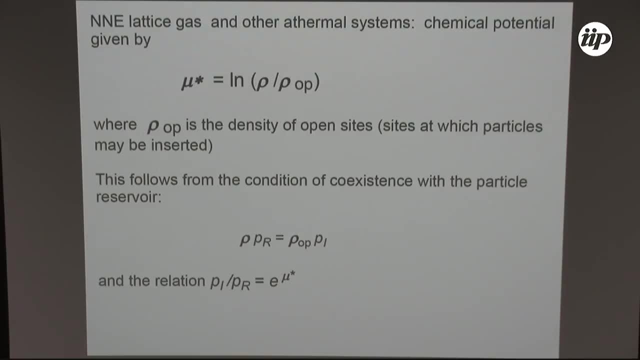 a number of events that allow each system in itself to forget about this interaction or this exchange. So we should expect this to work in what I call the weak exchange limit, or in other words, the rate of exchange attempts tending to zero. 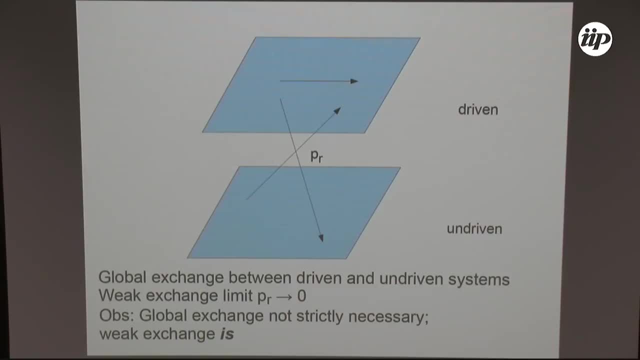 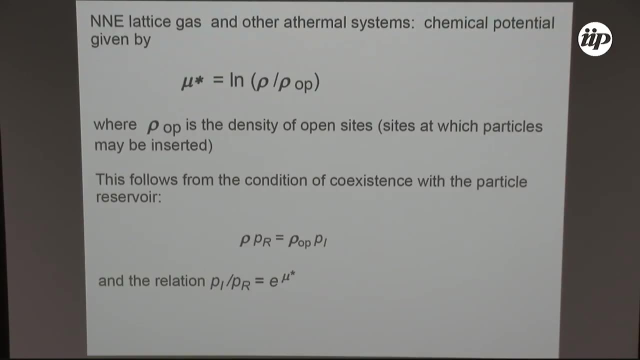 So that's shown symbolically here where I'm going to consider now. let's say I've done the following: I've run two systems, one with a drive, let's say with a strong drive, maximum drive- the other without any drive, for example. 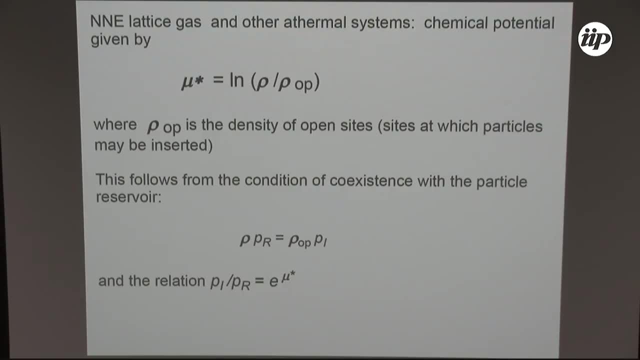 and I've done this calculation up top. I've determined to high precision the open site density as a function of the particle density. So now I have the chemical potential for this system in isolation. Now I'm going to allow exchange between these two systems. 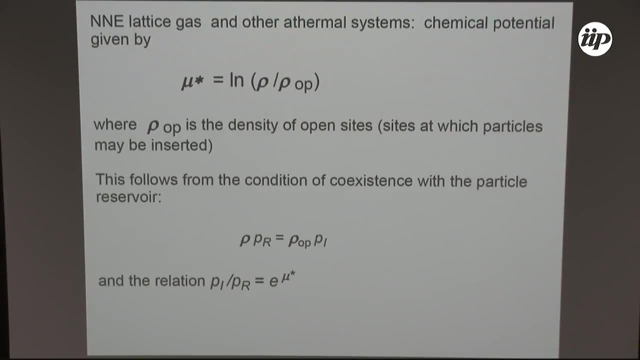 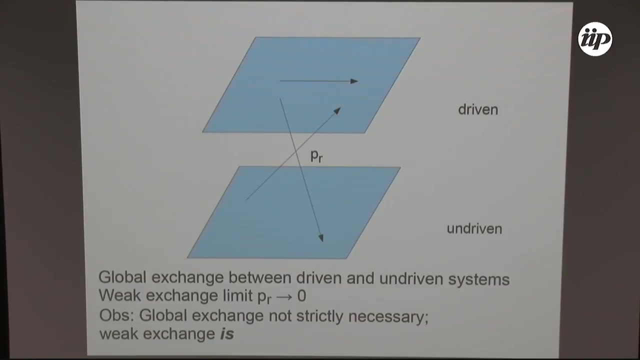 one that's in a non-equilibrium steady state and one that's in equilibrium, And I want to use my chemical potential to predict the densities in the two systems at coexistence. So the setup, symbolically, is this: The driven system exchanging particles with the undriven. 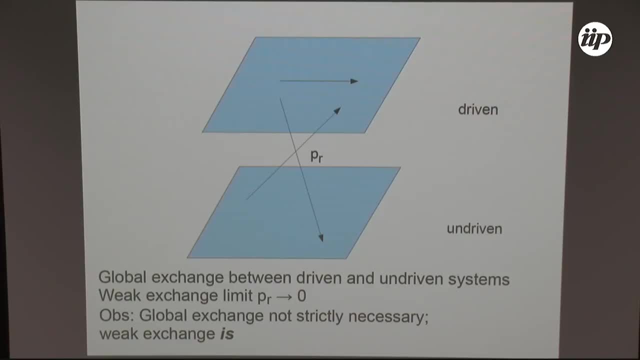 and there's this rate PR of exchanges. As a convenience this isn't necessary, but as a convenience I'll allow global exchange. In other words, a particle in any site in one system can hop to any other site. open site. 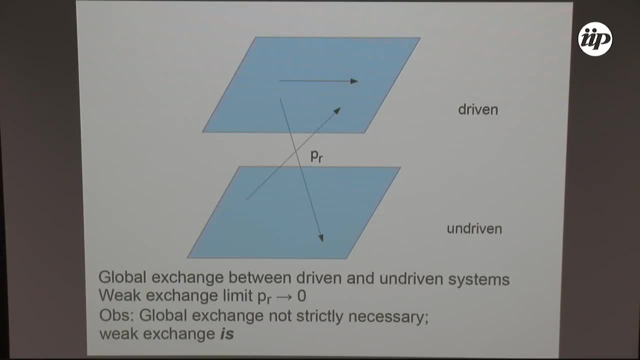 obviously in the other system. What this does is to minimize non-uniformities that would arise if I only allow exchange along an edge or along some restricted set of sites. But I can allow exchange only between a restricted set of sites. I just have to wait longer for the non-uniformities to disappear. 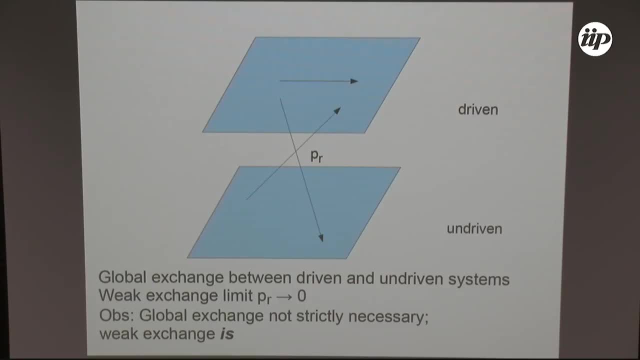 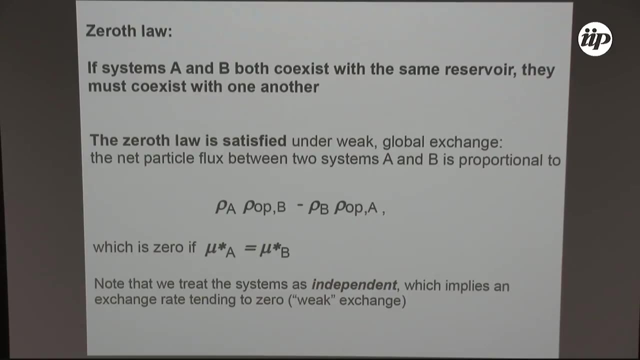 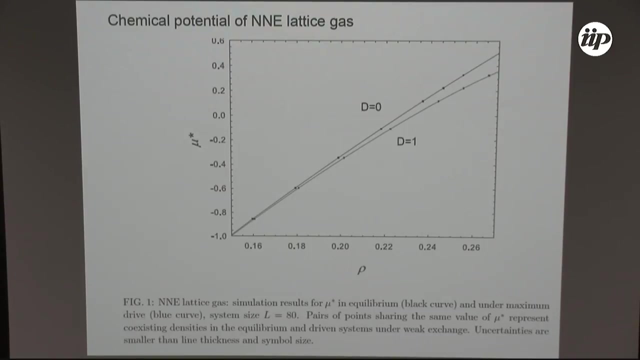 But the weak exchange limit is important. It's not optional. Okay, So this has basically been said already. Let me show you some results. This is from a square lattice of 80 by 80 sites and you see this chemical potential. 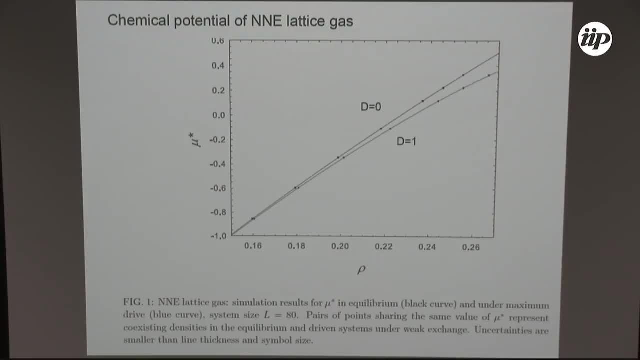 as a function of particle density: for the non-driven system, which is the upper curve, and for maximal drive, the lower curve. You also see pairs of points. The curves are obtained for the isolated systems, the two isolated systems. The pairs of points lie on a horizontal line. 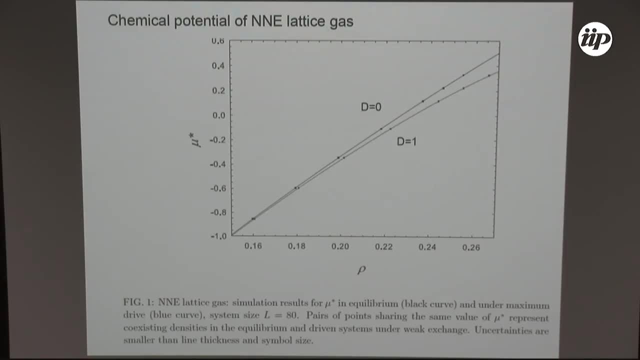 equal values of the chemical potential and they show the empirical densities obtained when the two systems are allowed to exchange particles. So we see that in this case, equating the chemical potential of the two systems really does predict the densities at coexistence. 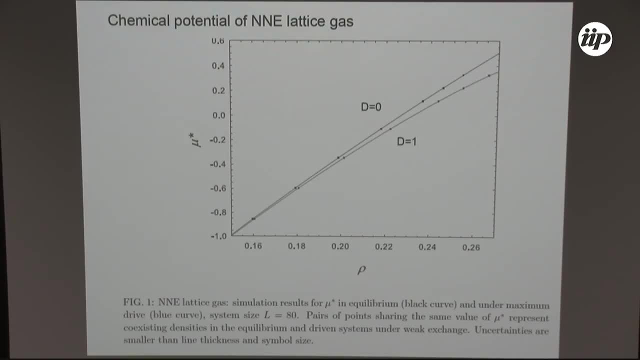 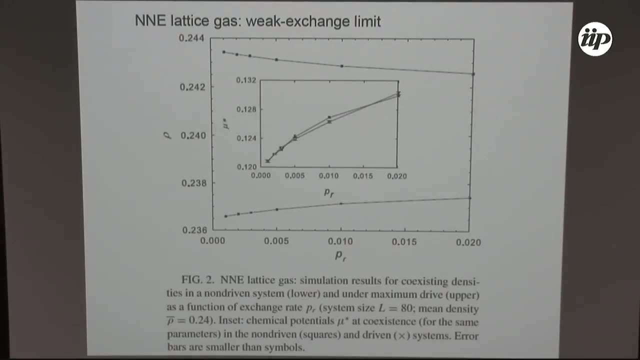 So it works the way you would like a chemical potential to work in thermodynamics. Here's a detail showing how the chemical potential, mu star, the inset, how it behaves as you reduce the exchange probability, the exchange rate, and you can also see in the main graph. 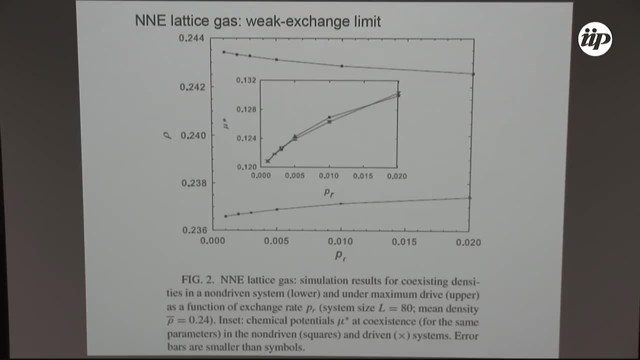 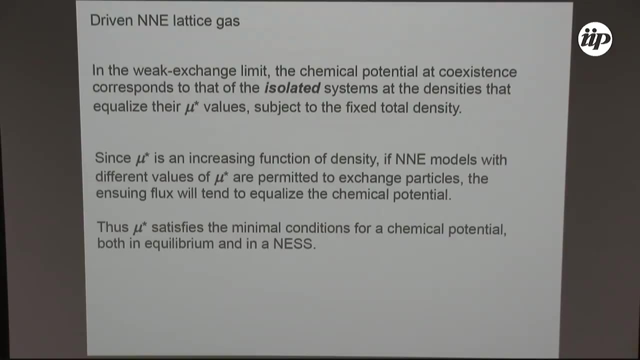 how the densities tend toward their limiting values, which are the values that equalize the chemical potential. So this worked, and I'm going to come back to this case at the end, but first I want to talk about this. I'm going to go very quickly. 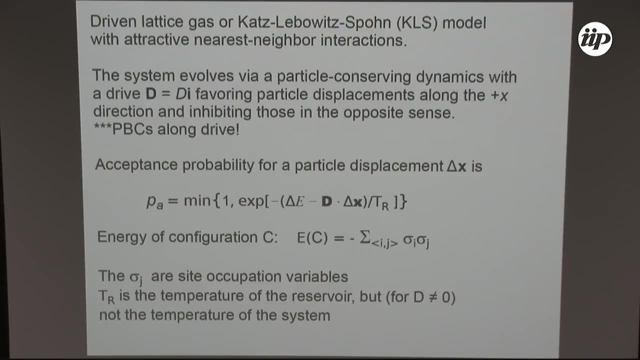 This is a model that may be familiar to people who've read about driven lattice gases, also known as the Katz-Lebovitz-Spohn model, in which you have a lattice gas with attractive nearest neighbor interactions, So now there's no nearest neighbor exclusion. 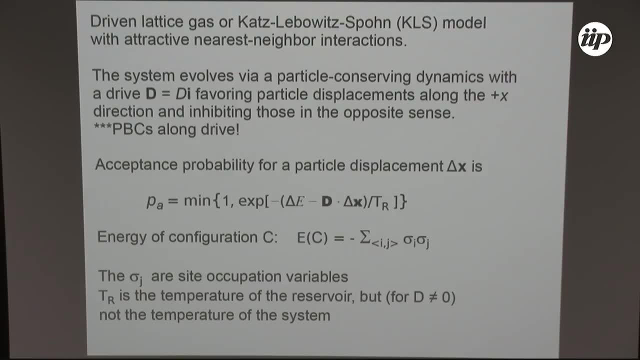 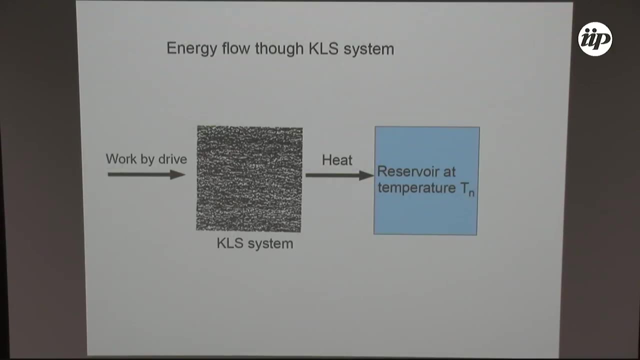 In fact, there's an energy function that looks like an Ising model, a nearest neighbor Ising model that favors clustering of particles, but you also have a drive. So this is another model that's been widely studied for non-equilibrium steady states. 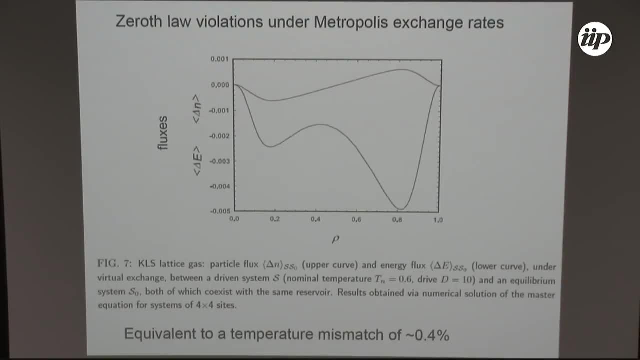 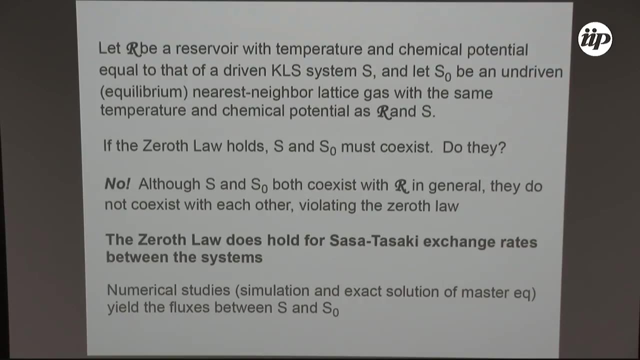 and all I'll mention about this is that it's possible to do this with the same thing as I showed before with chemical potential. Now we have to consider chemical potential and temperature, So a driven system will have its chemical potential defined via coexistence. 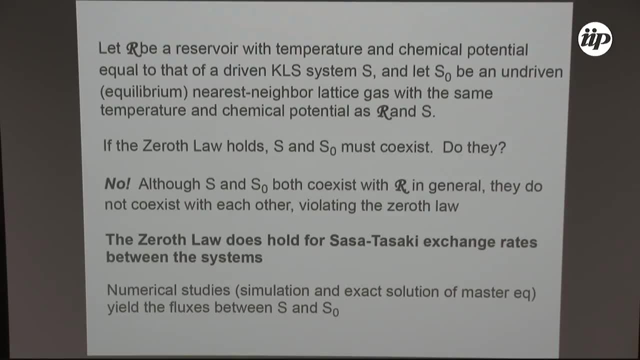 and also its temperature, again defined via coexistence with a heat reservoir. Again, you ask if these definitions of the intensive parameters obey the zeroth law, and the answer is that in general they don't, but they do for a specific choice of exchange rates between the systems. 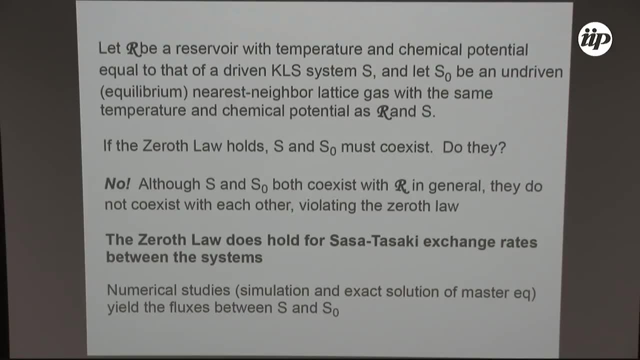 or between system and reservoir, which are the exchange rates that were defined by Saza and Tazaki in that article that I mentioned before. Basically, these exchange rates are like Cramer's problem: You have a particle sitting in a potential well. 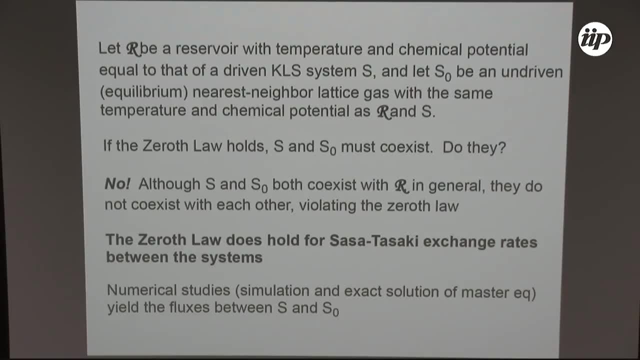 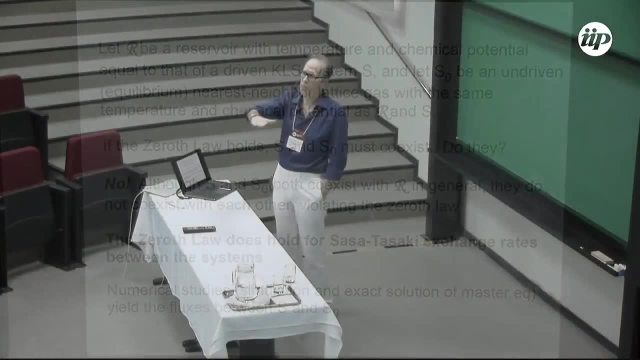 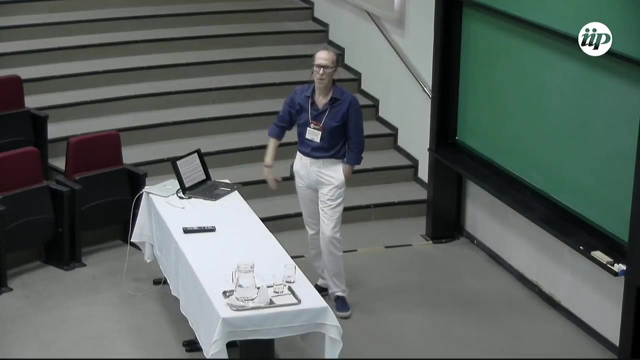 and it wants to get over the hill to the lower potential. well, but it doesn't know what's on the other side of the barrier. So these rates only involve the energy barrier between where the particle is now and where it has to get in order to go on. 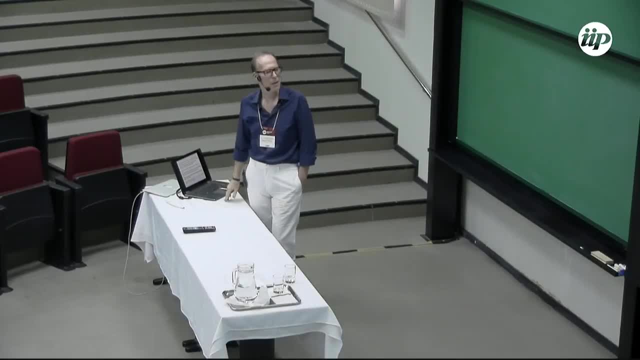 So they're not the same as metropolis rates that everyone likes to use in simulations because they're more efficient, but in some sense they're more physical. In any case, for this choice of rates it's possible now to define for systems with an energy scale to the interactions. 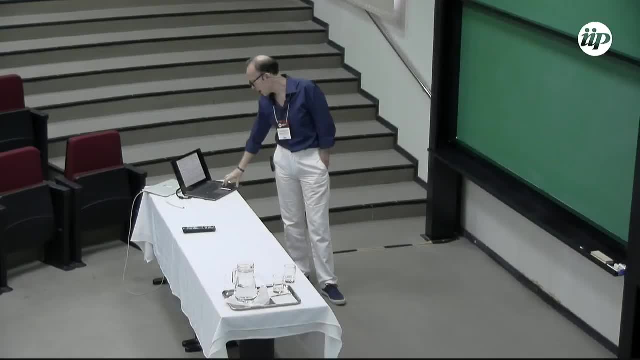 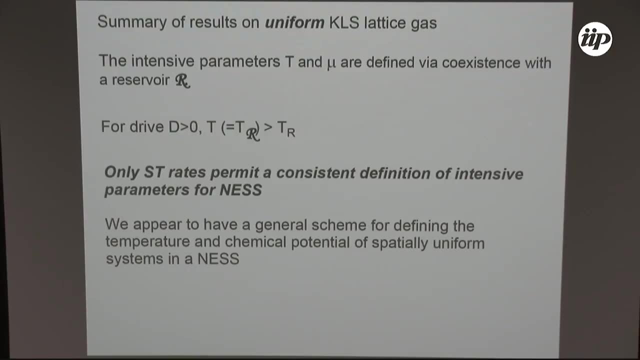 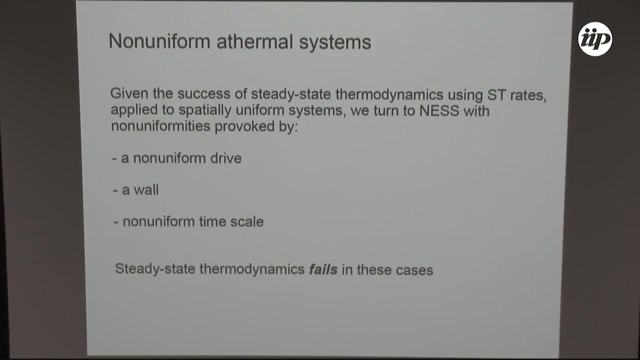 it's possible to define a temperature, And it all works as long as the systems are uniform. It fails when the systems are not uniform. So, very quickly, I'll show you a case where it doesn't work. I'm going to go back to the lattice gas. 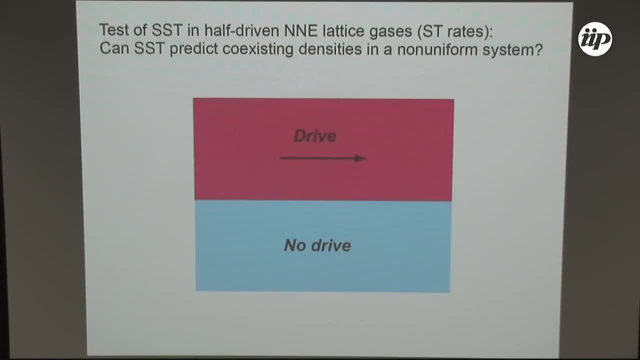 with nearest neighbor exclusion, And I'm going to take my lattice and simply apply the drive in half the system. So half the system the rates are skewed the way I showed and in the other half of the system they're symmetric. So I can think of this as a system that's split in half. 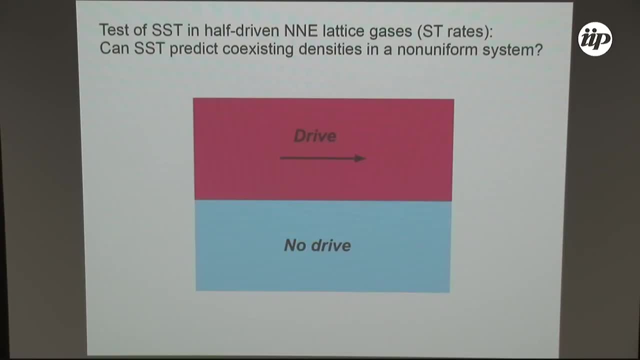 or I can think of it as two systems that, in their non-equilibrium system, in their steady state, will coexist. Of course, particles are allowed to hop across the boundary, and so we should expect them to coexist in the stationary state. Now, the idea is that it should be possible. 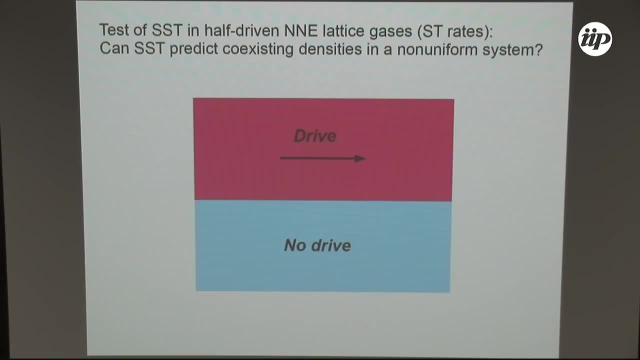 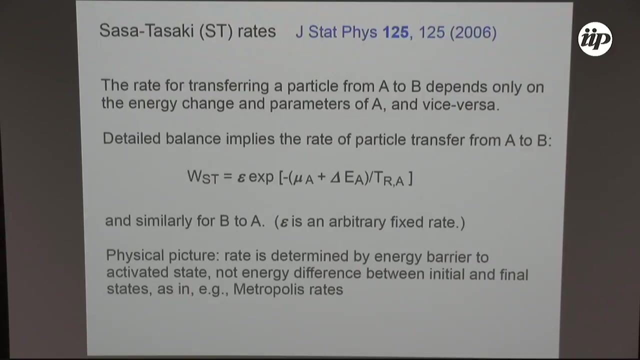 to use the chemical potential functions that I've shown you before to predict the densities of the two coexisting systems, one driven, the other not. And remember that the chemical potential just running back to this picture for a second, the chemical potential in the driven system. 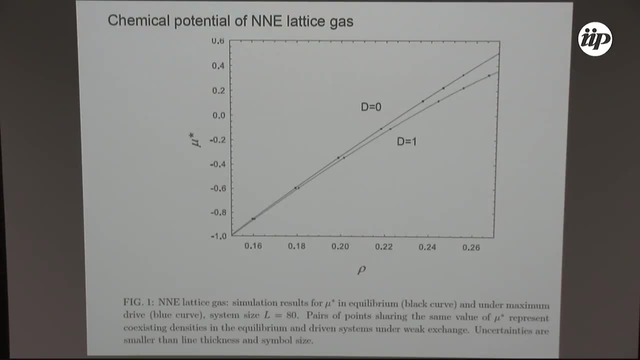 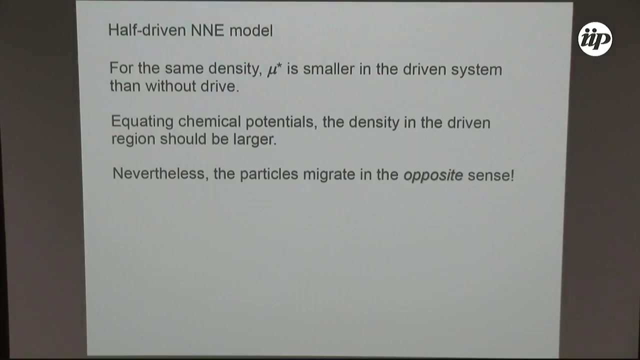 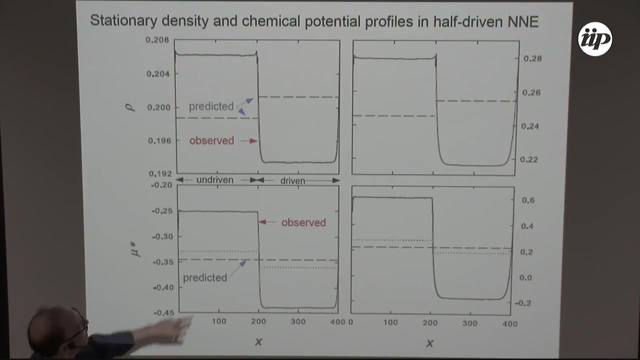 is smaller than in the non-driven system. So when I put these two into contact, I would expect particles to migrate from the non-driven to the driven, equalizing the chemical potentials. What actually happens is exactly the opposite: The particles migrate from the driven to the undriven. 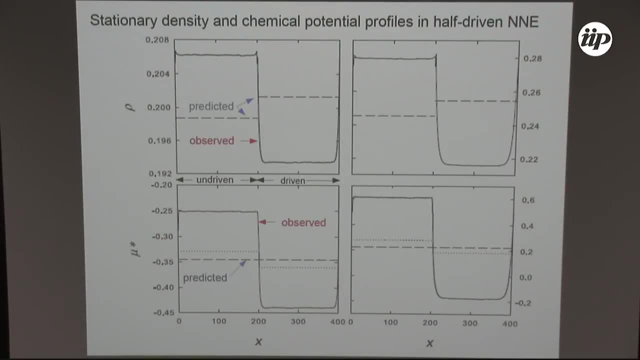 This curve is showing the density profile, the regions that are undriven and driven. The dashed lines are what is predicted by equating the chemical potentials, and the solid line is what you actually see. So it's one example. There are other examples where you can see. 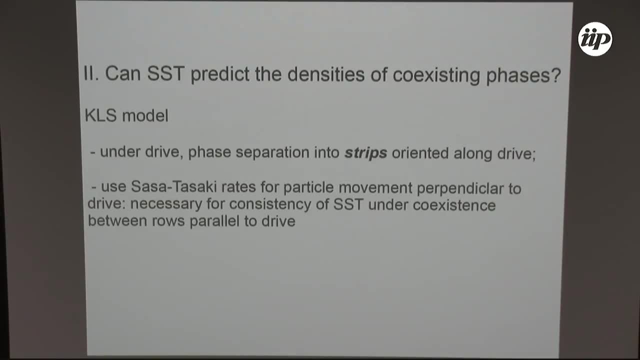 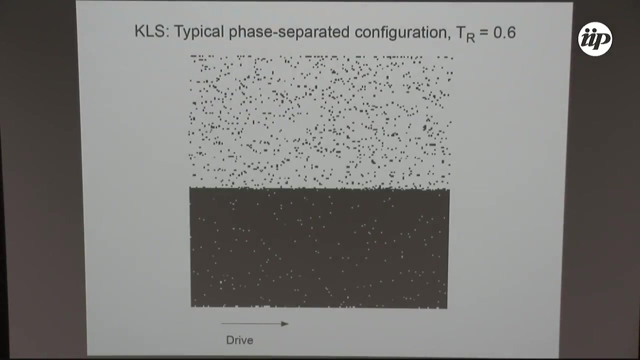 this kind of failure- Putting in a hard wall, for example- is enough of a perturbation to the uniform state that you see violations. I won't go into all of them. Okay, What about coexisting phases out of equilibrium? Let's look at this driven lattice gas. 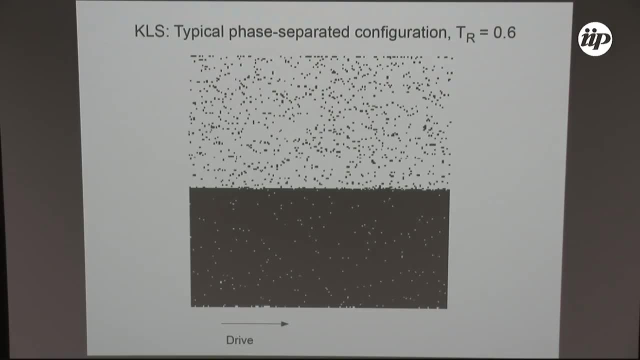 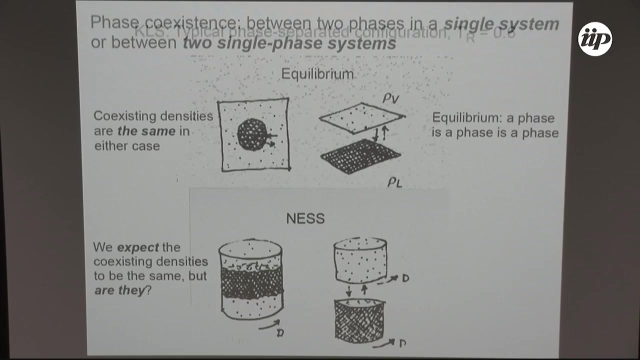 the KLS model, which does exhibit a transition, let's say a liquid vapor phase transition, at a certain temperature. Here we're well below the critical temperature, so we see a strong density contrast. But the question I want to ask is the following: 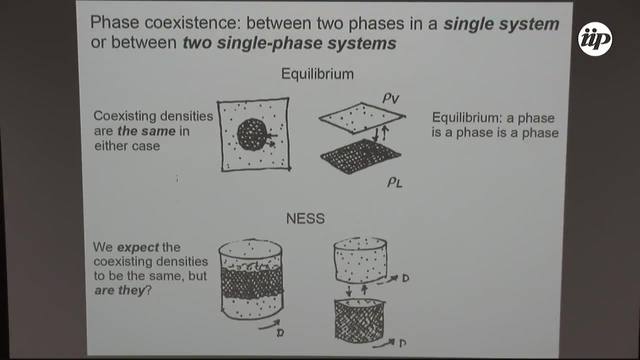 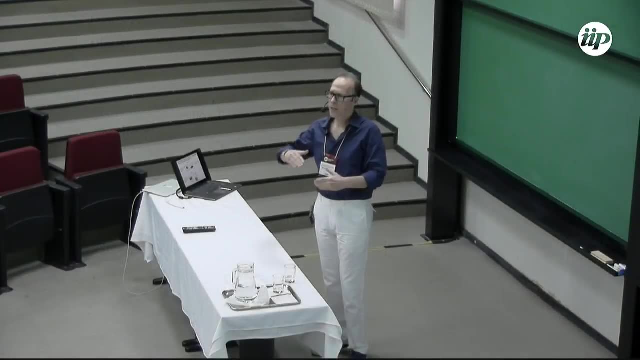 In equilibrium. we can have phase separation in a single system or we can take two phases and have them in separate systems and allow exchange. So we can have two phases of particles of energy between these two systems that are in pure phases And we know that the properties 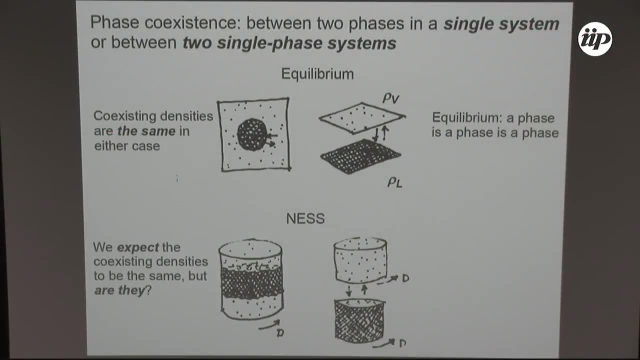 at a given temperature and other conditions being equal. the properties of the two phases that are separate, pure phases but that exchange particles and energy between them, those properties are exactly the same properties in a phase separated system, where I have macroscopic samples of the two phases. 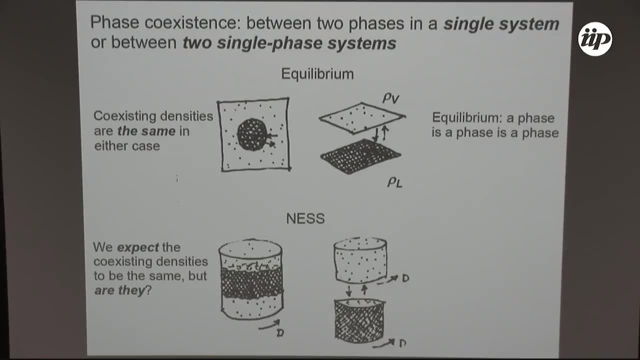 So I'm going to ask if the same thing happens in non-equilibrium steady states. I'm going to do this in the driven lattice gas with nearest neighbor interactions at a temperature such that there is phase separation. So I take my system symbolically here a cylinder. 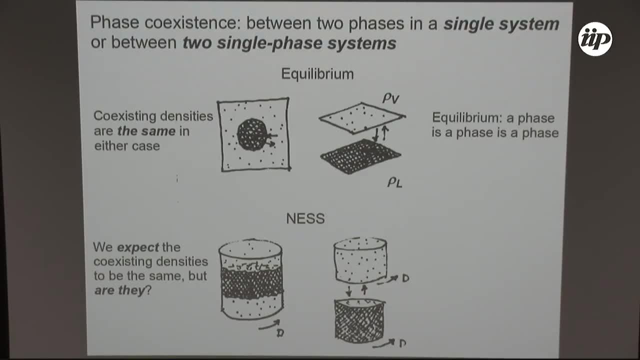 with the particles running around the periodic direction and below the critical temperature, I observe phase separation, more or less as I showed you in that picture. I can also take two separate systems and adjust the densities to be equal to the densities observed here. Initially they're separate. 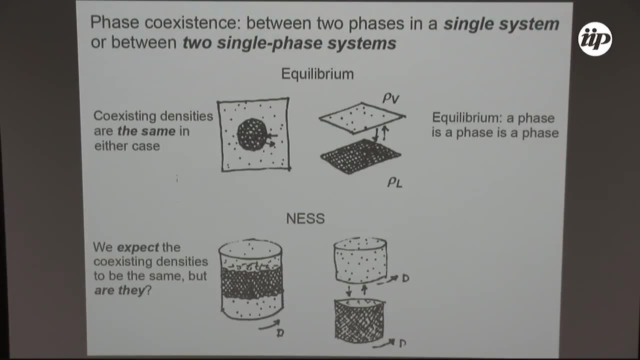 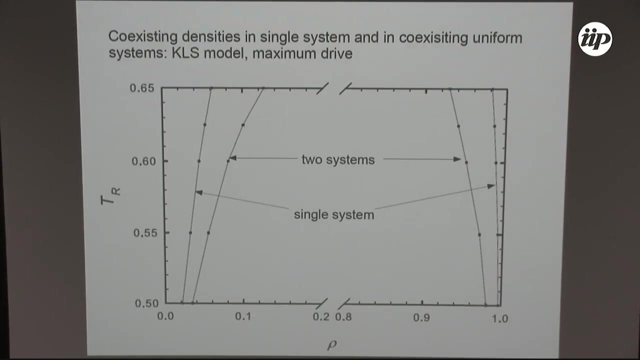 Now I let them reach their respective non-equilibrium steady states and I start allowing them to exchange particles at a slow rate. Do the densities stay the same as they were here initially? The answer is no. In fact, the temperature density diagram is quite different. 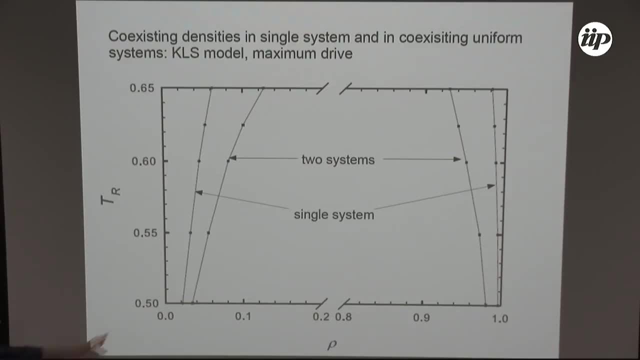 for the single system that's phase separated spontaneously, and for the two systems that are in pure phases but that are able to exchange. So without going into details of definitions, in this case of chemical potential and temperature, you see that we're going to have problems. 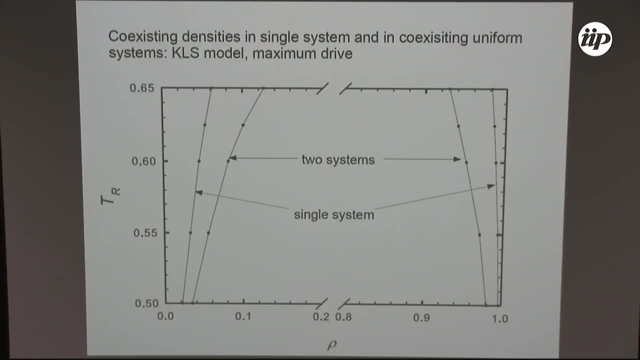 using any scheme of steady state thermodynamics to predict phase coexistence, because the usual game is to determine intensive properties in isolated systems and then equate these properties to predict what happens when systems phase separate, or vice versa. But here it just doesn't go through. 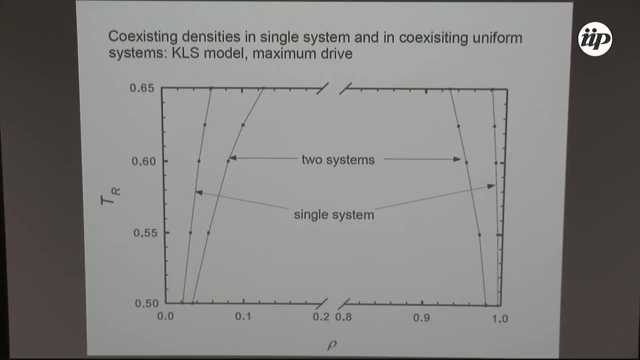 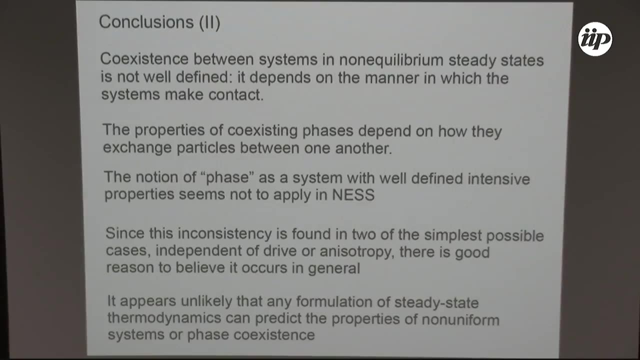 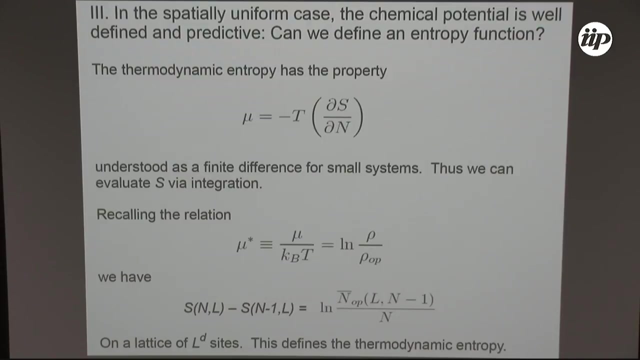 So another problem with steady state thermodynamics. How much time do I have left? Five minutes, That's good. So now let's look at the entropy. Let's go back to the case of the uniform driven lattice gas with nearest neighbor exclusion, where it was possible. 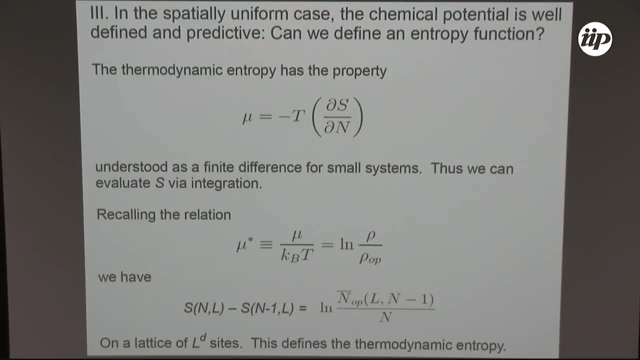 to define a chemical potential and verify the zeroth law, verify that it has some predictive power. Well, if you have a chemical potential, you should be able to have an entropy. So that's just. I mean, basically, it's a question. 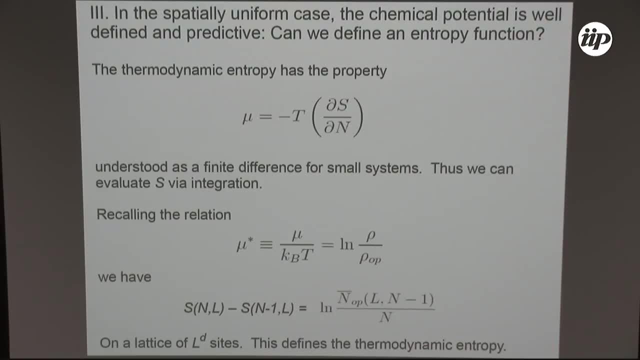 of thermodynamic integration. So since we're in small systems, you have to interpret that classic definition as a finite difference. but you do that here. So I have two systems of the same size. I'm changing the number of particles by one. 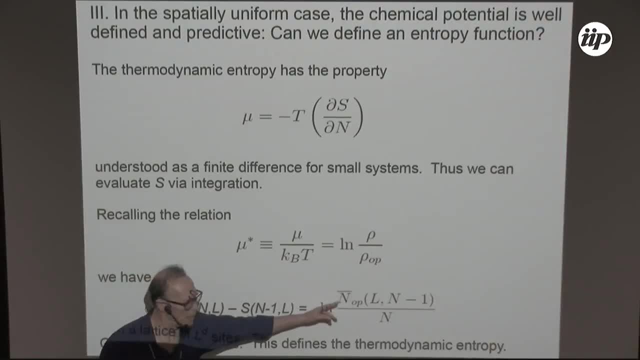 and I look at the change of entropy and, going back to our definition of chemical potential, it leads to this simple relation. So that's our definition. Okay, nothing new here. but I'm going to ask the following question: Is this the Shannon entropy? 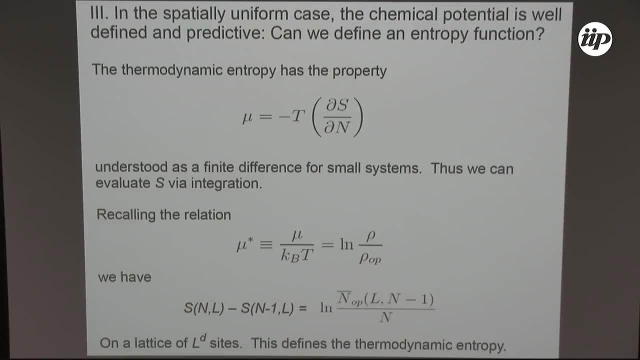 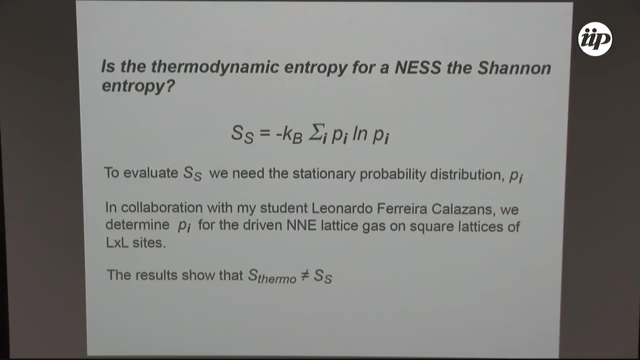 To answer that question, of course I have to know the stationary probability density. That's not so easy. I can't really get the stationary probability density in Monte Carlo simulations, but I can take the master equation and for systems that aren't too large, 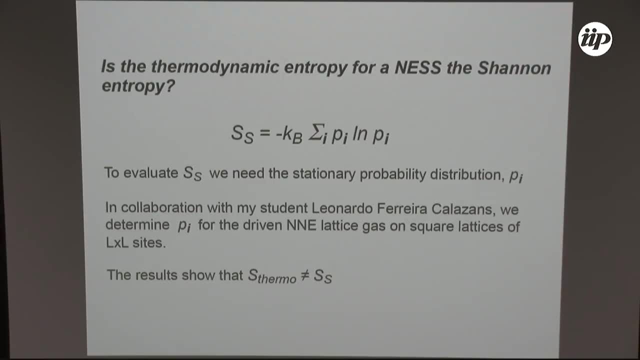 I can use an iterative method to find the stationary probability density. So what we've done, along with my student Leonardo, is for systems of size up to six by six sites, so a decent-sized system. I mean it's very small. 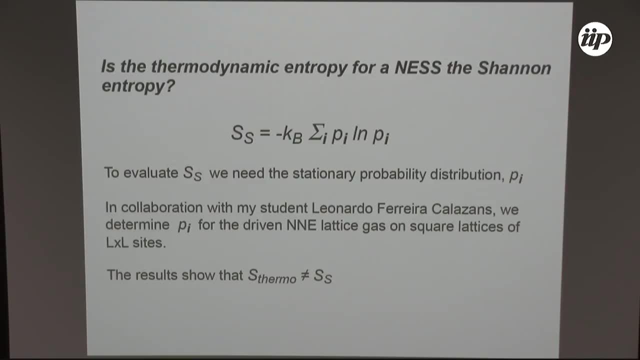 but it's large enough to show some interesting behavior, and the space of the surface is not too big, It's very, very small. So that's the question. So what's the stationary probability density? Well, this is a very complex question. 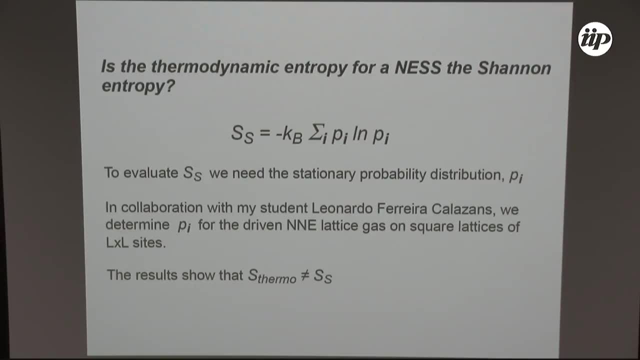 There are a number of different configurations already contains on the order of a billion configurations for certain cases. So we can find the stationary probability density and calculate the Shannon entropy and compare that to what I'll call the thermodynamic entropy, in the sense that we predict. 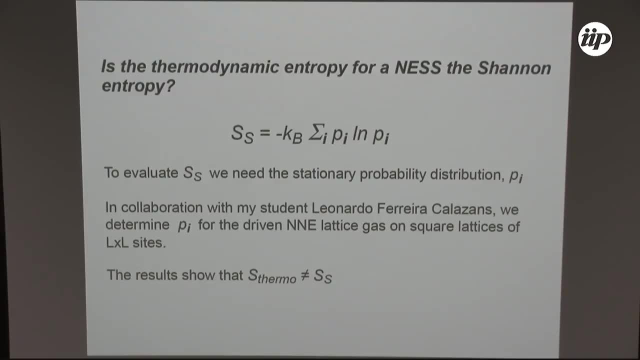 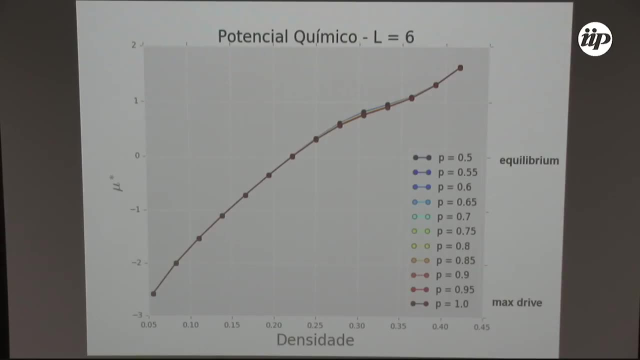 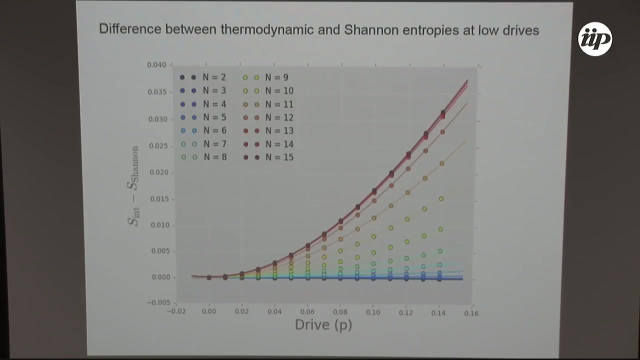 properties at coexistence. And the fact is that the two are not equal. So who cares? Well, oh, here are some results. So here are some numerical results, not simulations, but from this iterative solution of the master equation showing you: 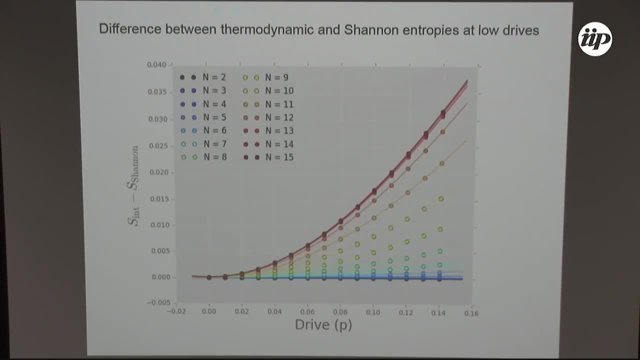 how the difference between the entropy and the stationary density and the Shannon entropy that was obtained using the integration formula and the Shannon entropy differ, As you would expect, for of course, for drive zero they have to be the same, but for weak drives the difference.